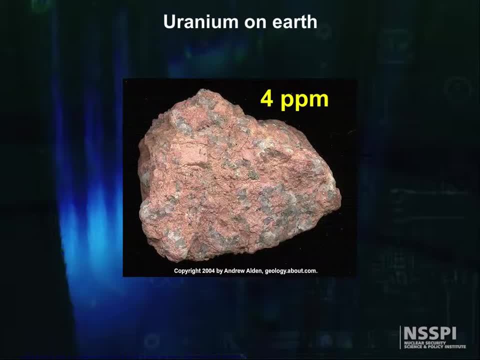 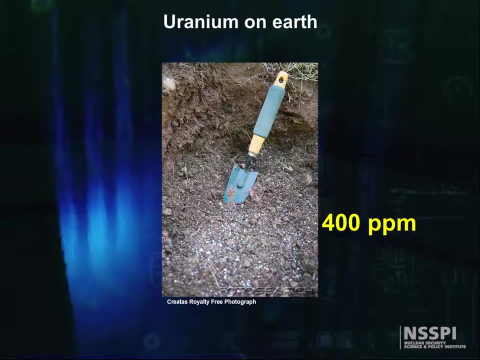 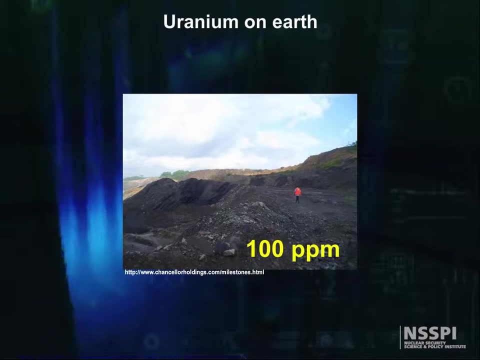 and since granite makes up 60% of the Earth's crust, you can see that it's everywhere. Fertilizers contain uranium concentration as high as 400 parts per million, which makes them almost an ore body, And some coal deposits contain uranium concentrations greater than. 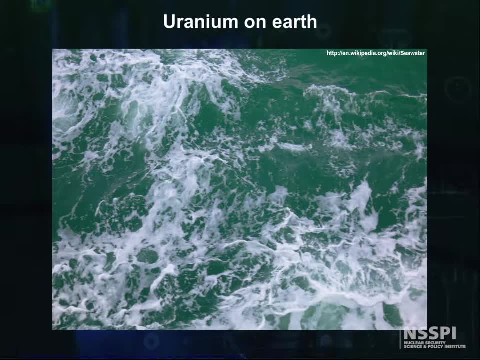 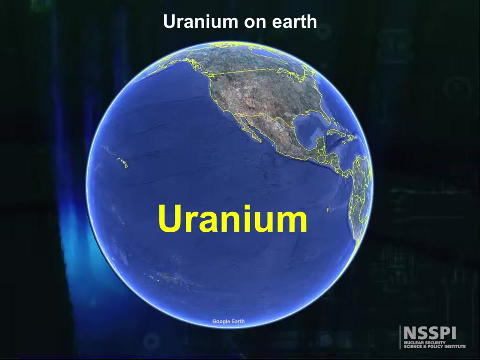 100 parts per million. Seawater contains approximately 3.3 milligrams of uranium per cubic meter. That's 3.3.. This resource is gigantic If recoverable. this amount is limitless compared to the world demand. If even a portion of uranium in seawater could be used, the entire world's nuclear 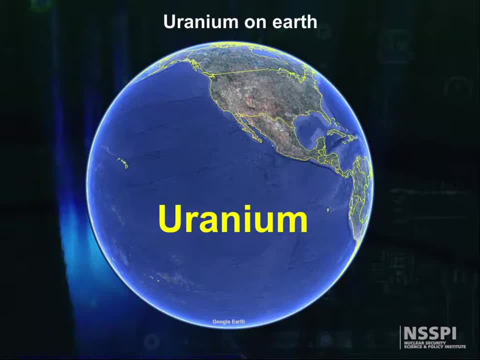 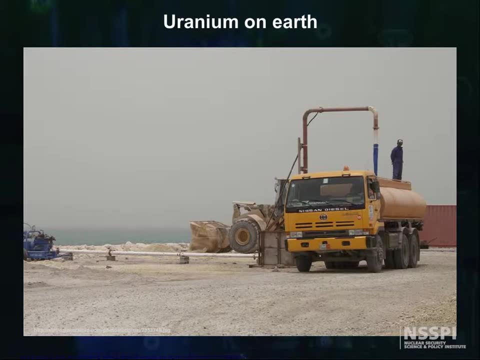 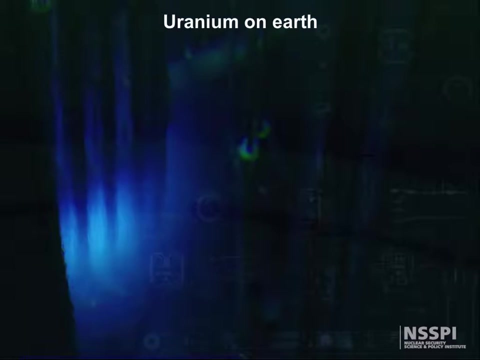 fuel for power generation could be provided for thousands of years. Well, so as not to tell a part truth, if the seawater has to be pumped more than a few feet in height, the pump work is more than the energy that can be recovered from the uranium. 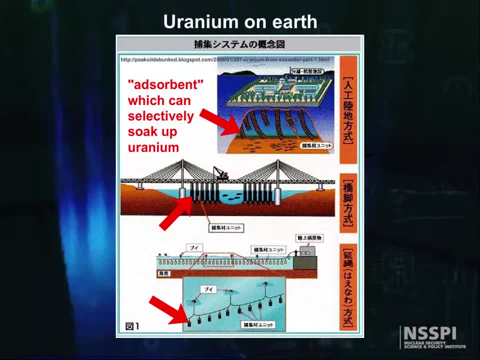 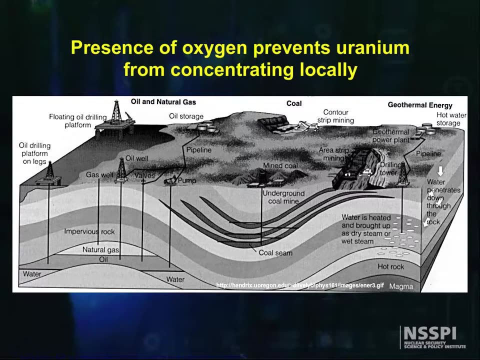 To end on a more positive note, by using tides and new recovery techniques worked out in the last few years, uranium from seawater is probably within a factor of two or so from being economically feasible. Back on land, it's the chemistry of uranium that usually prevents it from concentrating. 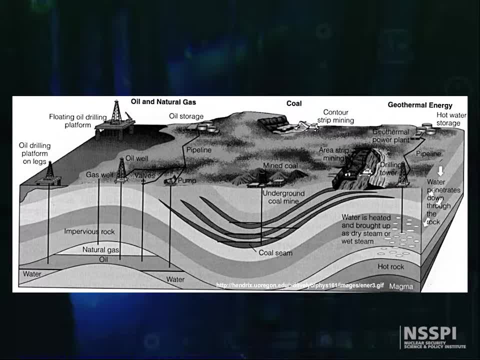 locally. It's the chemistry of uranium that usually prevents it from concentrating locally: It's just too soluble in the presence of oxygen. However, geologic anomalies have occurred at a number of places around the world so that the concentration of uranium there is sufficiently high that mining is economically 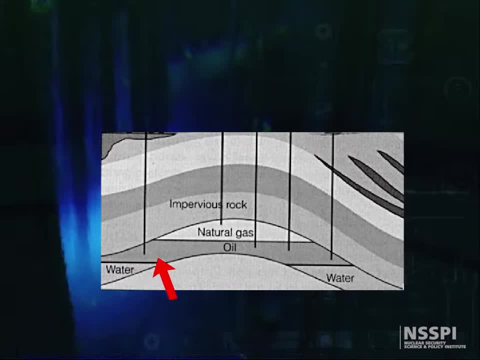 feasible. These anomalies usually consist of places where oxygenated groundwater carrying uranium met with a reducing agent such as percolation. That's why uranium is so soluble in the presence of oxygen. That's why uranium is so soluble in the presence of oxygen. 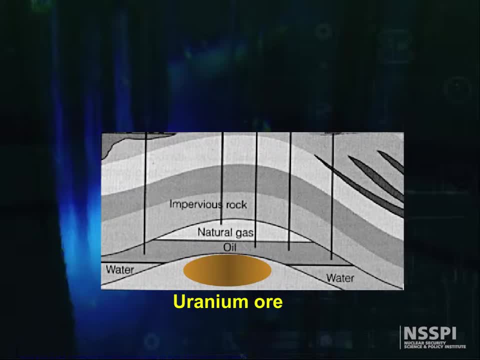 All it takes is petroleum deposits buried wood or peat. All it takes is petroleum deposits buried wood or peat. The uranium is reduced and the valence. four compounds are insoluble and deposit at the reduction site. In the absence of oxygen, the deposits are geologically stable. 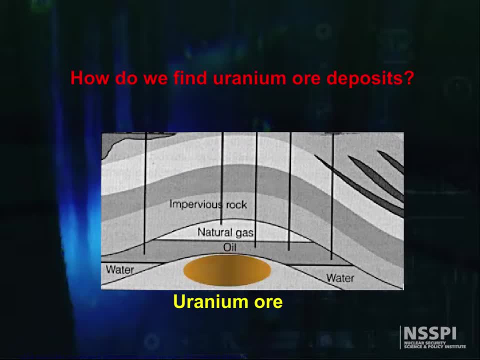 In the absence of oxygen, the deposits are geologically stable. Well, how do we find these uranium ore deposits? Uranium prospecting is pretty much the same as other mineral exploration, except for the specialized instruments that exist for detecting the presence of radioactive ores. 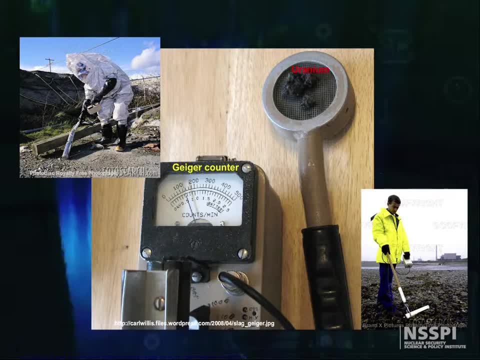 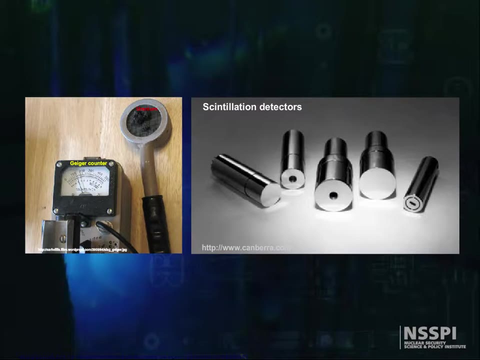 The Geiger counter was the original radiation detector and was the principal instrument used for uranium prospecting for many years, until Geiger counters were replaced by scintillation counters. Scintillation counters are 10 to 1,000 times more sensitive than Geiger counters. 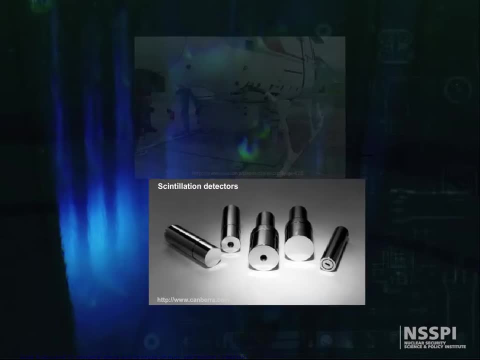 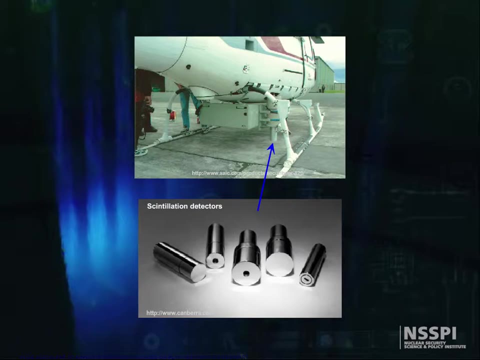 In the late 1940s, several folks had the bright idea to put these scintillation detectors on airplanes and look for deposits from the air. Airborne gamma ray detection is now the leading technique for uranium prospecting. A deposit of uranium discovered by 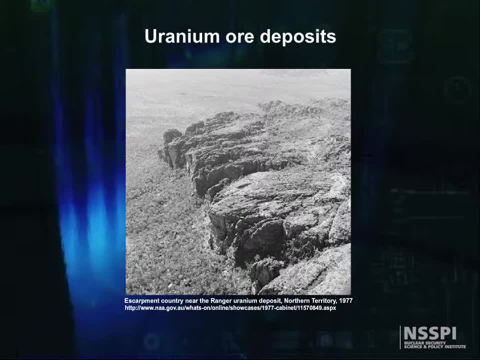 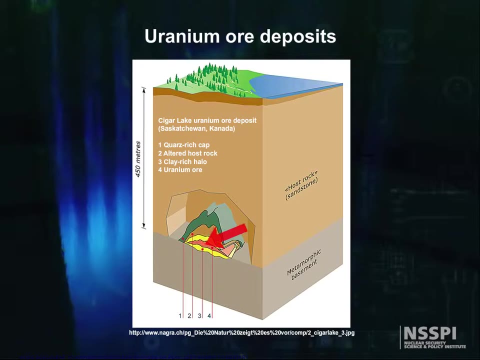 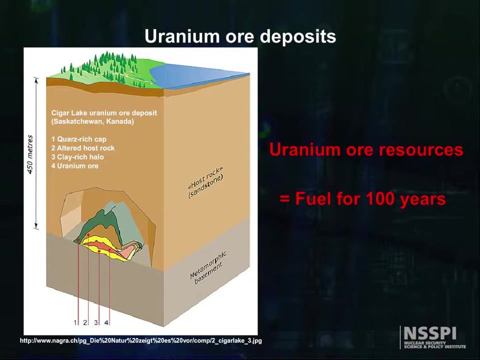 geophysical techniques is evaluated and sampled to estimate the amount of uranium that could be extracted at specified cost. Uranium reserves are the amount of ore that are estimated to be recoverable at specified cost. Known ore resources which can be mined at about the current cost. 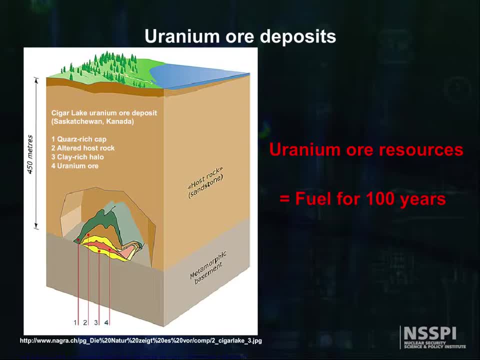 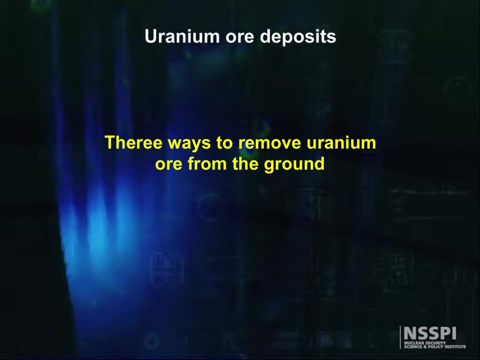 are estimated to be sufficient to provide fuel for about a thousand tons of uranium. Uranium is estimated to provide 100 years, based on the 2006 nuclear energy generation rate. Uranium ore is removed from the ground in one of three ways, depending on the location of the deposit. 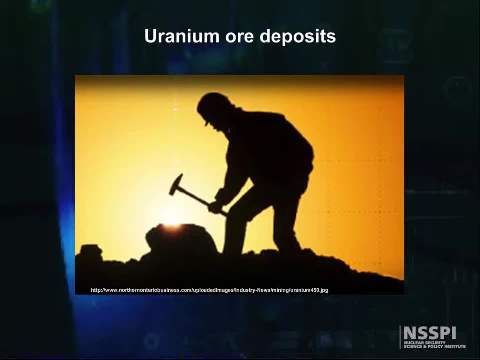 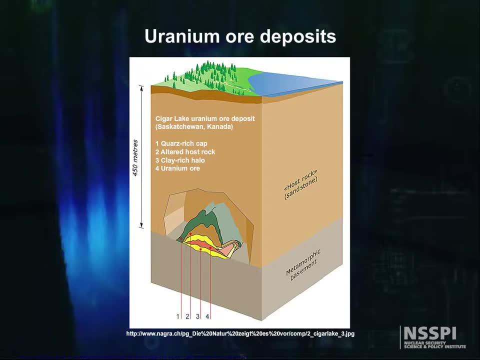 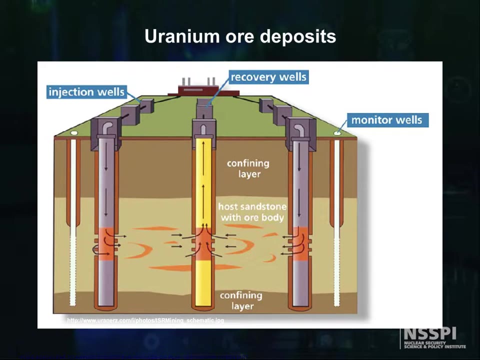 Uranium deposits close to the surface can be recovered using the open pit mining method, and underground mining methods are used for deep deposits. Sometimes the ore may be extracted from the ground, and the ore may be extracted by in-situ recovery, a process that dissolves the uranium while still underground.